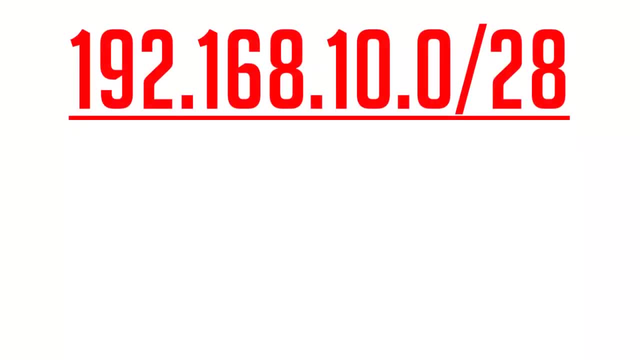 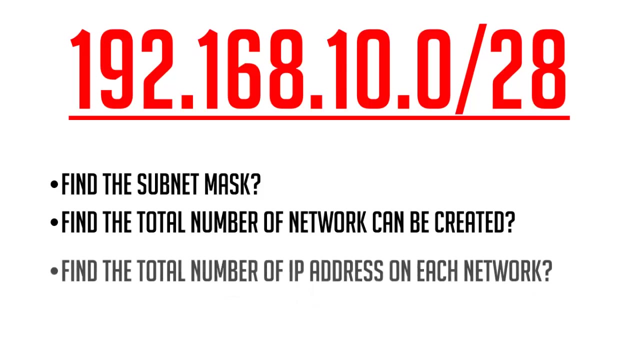 Hello friends, in my previous video of subnetting I have asked you one simple question. that is from 192.168.10.0 with the CIDR value 28,. find the subnet mask. Find the total number of network can be created. Find the total number of IP address on each network and find the total number. 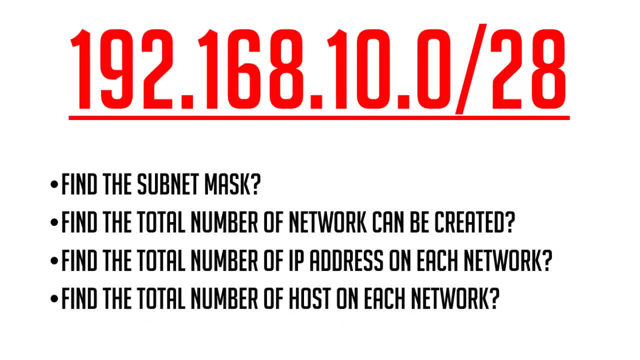 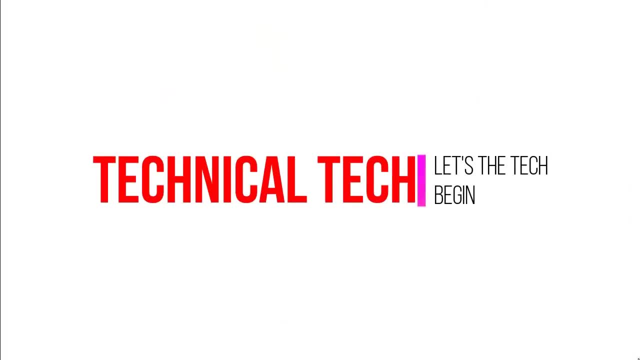 of host on each network. In this video, I am going to explain you how to find the answer of this question. Hello friends, this is Abhishek here and welcome back to my channel, Technical Tech. Let's the Tech begin, As here you can see, the IP address starts from 192.. It indicates it is a. class C IP address. The default subnet mask of class C IP address is 255.255.255.0.. This is because, by default, there are 24 bits are reserved for the network And 8 bits are reserved for the host. So once you calculate these binary bits on each block. 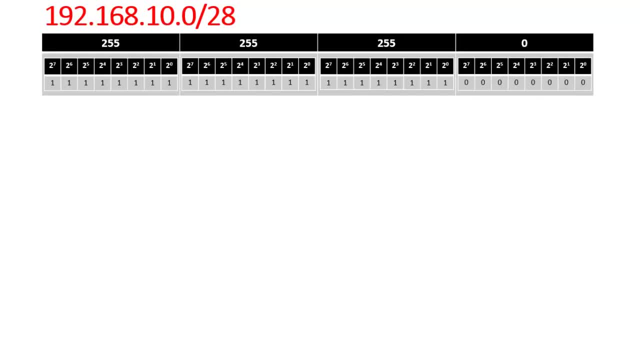 you will get 255.255.255.0.. But the question is here: the CIDR value is 28.. And by default the number of network bits on class C IP address is 24.. So from where do we get another 4 bits? 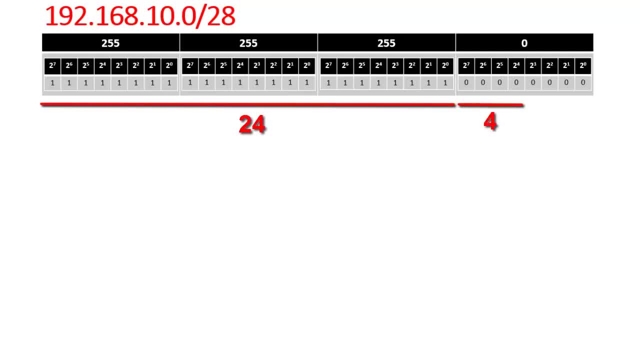 That is, we have to borrow 4 bits from the host to make it 28.. So the new subnet mask. what you will get is 255.255.255.240.. Now from where do we get this number 240?? This number is the value of. 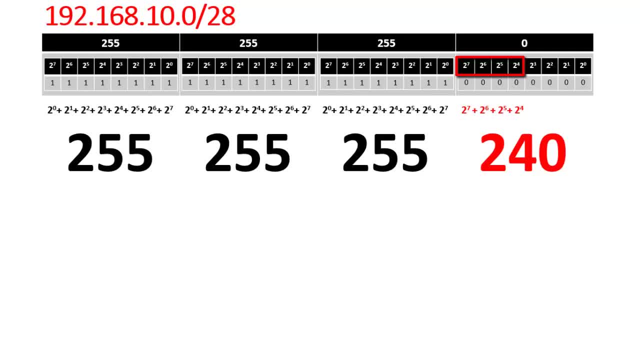 bits which you have borrowed from the host, As here you can see: the value of 8 octet is 2 to the power 7, plus the value of 7th octet is 2 to the power 6, plus the value of 6th octet is 2 to the power 5, and. 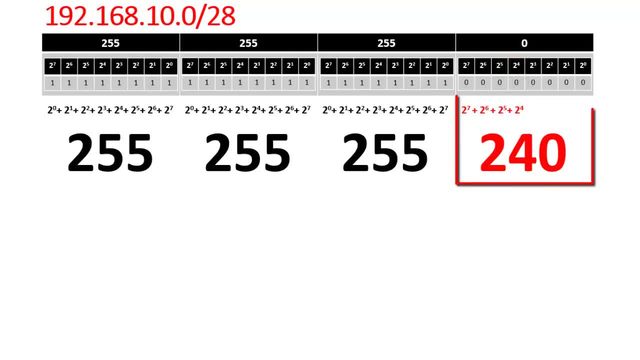 octet is 2 to the power 4.. Once you calculate all these values, the total number you will get is 240.. So the subnet mask of 182.168.10.0 with the CIDR value 28 is 255.255.255.240.. Is it clear, guys? 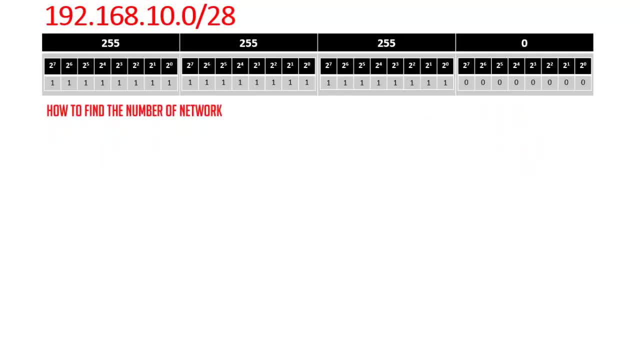 Now let's find how to find the number of network. I have explained everything in my previous video, So if you have not yet that video, so please watch it, because i have explained you each and everything from basic to advanced level. i will highly recommend you to watch that video too. okay, now let's find the 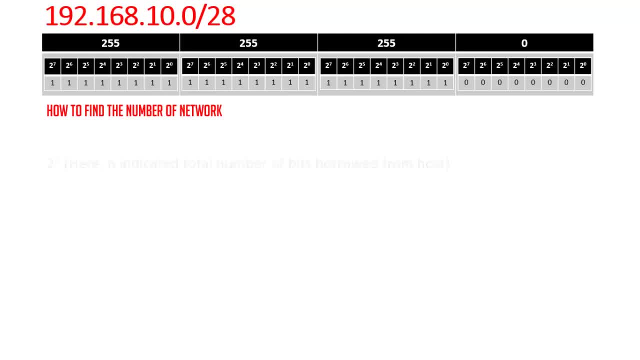 number of network from this address. so what is the formula for this? it is 2 to the power n. here n indicates the total number of bits borrowed from the host. so how many bits we have borrowed from the host? we have borrowed 4 bits. so what will be the answer? it will be 2 to the power 4, which. 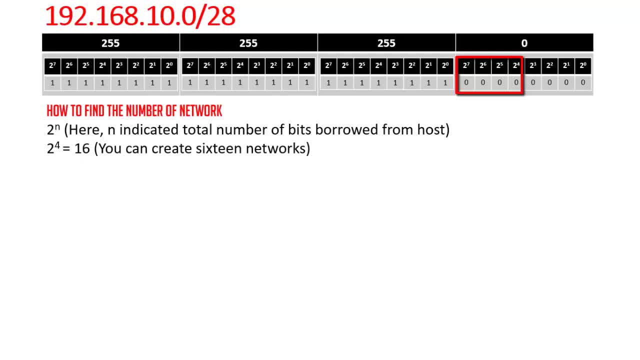 is equal to 16, it means you can create total number of 16 network from this address. now how to find the number of ip address on each network? so the formula is very simple. again we have to write it. 2 to the power n, but in this scenario, here n indicates the total number. 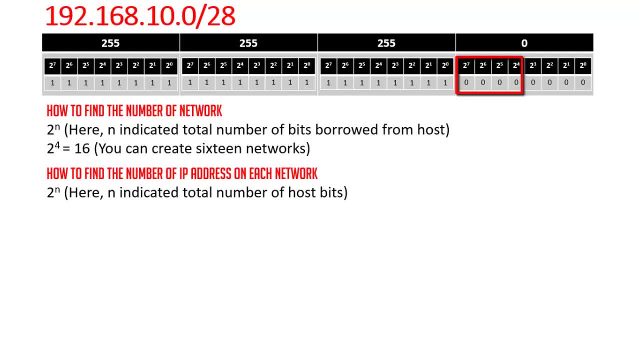 of remaining host bit. we have already borrowed 4 bit. okay, now how many bits remaining to the power? 4 so, which is equal to 16. it means on each network you will have 16 ip address. now how to find the total number of host on each network? hence the formula is quite similar: it is 2 to the power. 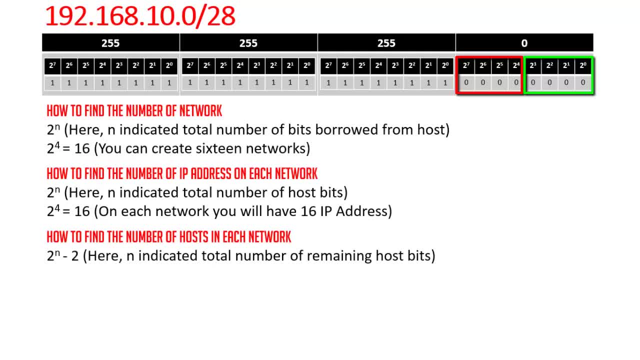 n minus 2. here n indicates the total number of remaining host bit. so how many bits remain in the host part? that is 2 to the power, 4 minus 2, which is equal to 14.. you will have total number of 14 host ip address on each network. now the question is why we have 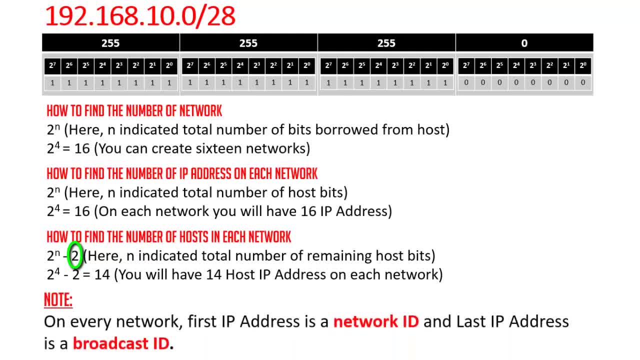 subtract 2 here. this is because on each network the first ip address is reserved for the network id and the last ip address is a broadcast id. so how many ip address remained? remained only in ip address, and this will be the host ip address which is assigned to the pc. 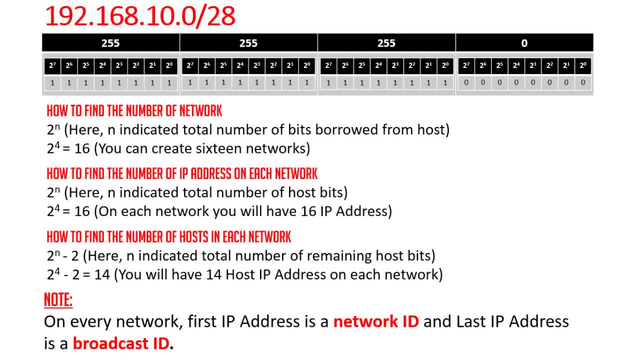 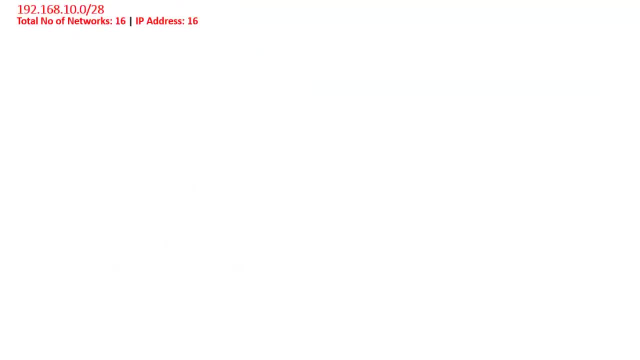 now i am going to show you the table where i have mentioned the network id, host, i address and the broadcast id of each network. so hence the total number of network. what we have found is 16 and total number of ip address on each network we have found is 16.. 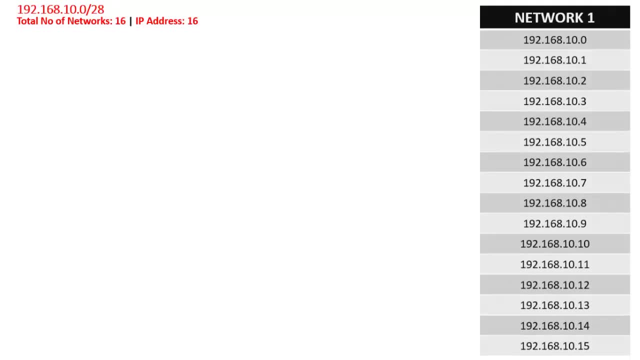 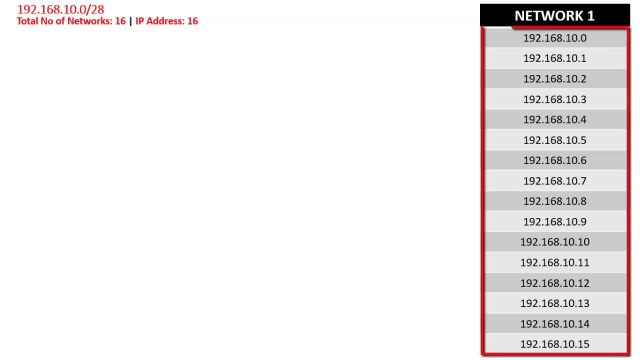 okay, it is 16- 16.. now in network 1, the ip address will start from 192.168.10.7.. 0 to 192.168.10.15. there are total number of 16 ip address on each network, even in network 1. 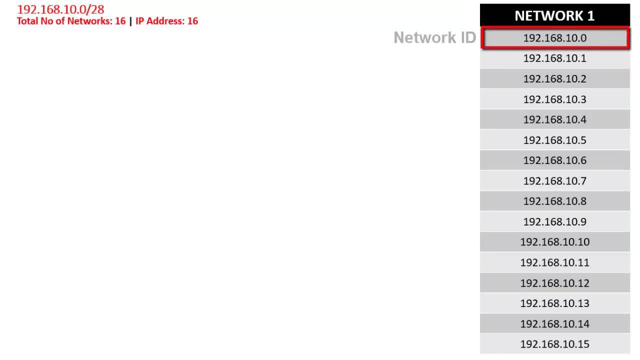 it is 16 ip address, so the first ip address is a network id and the last ip address is a broadcast id. so how many ip address remained here? there are total 14 number of ip address are remaining, so this is the host id. here is a table. here i have mentioned the network. i 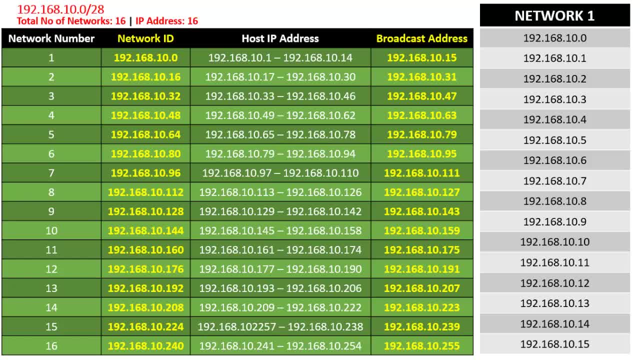 have mentioned the network id and the last ip address is a network id, so you can check this table. so, guys, this is all about today. i will highly recommend you to watch my previous video, guys, because that is very simple: if once you watch that video, your all the doubt. 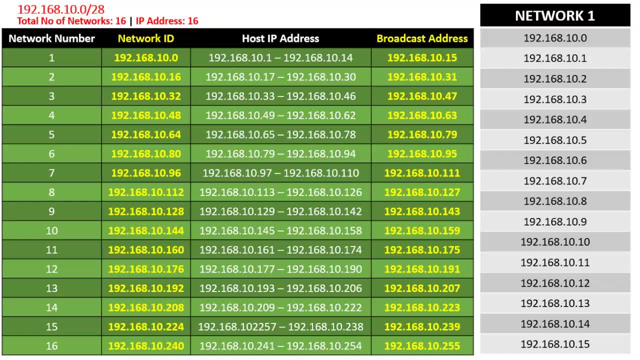 and the confusion will be clear. i will provide you the link of that video in the description section below and by watching that, please let me know how is the video and how is your experience. if you are having your doubt, any doubt, please let me know in the comment section. 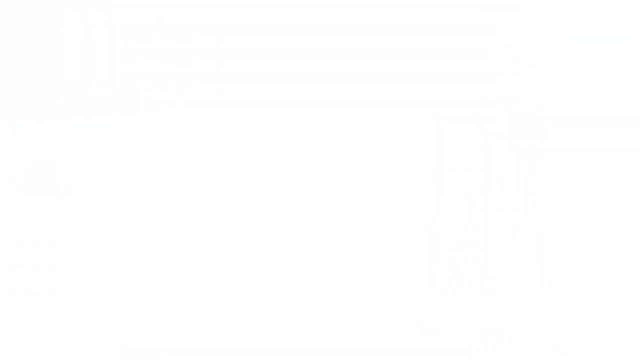 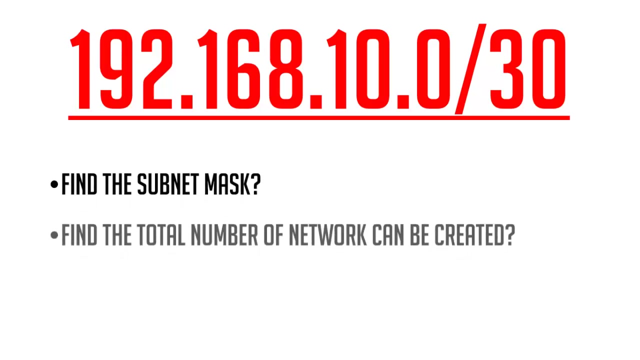 below. i will answer it for you, will try to help you guys. so, guys, it's time for the surprise test and today's question is from 192.168.10.0, with the CIDR value 30. find this subnet mask. find the total number of network can be created. find the total number of IP. 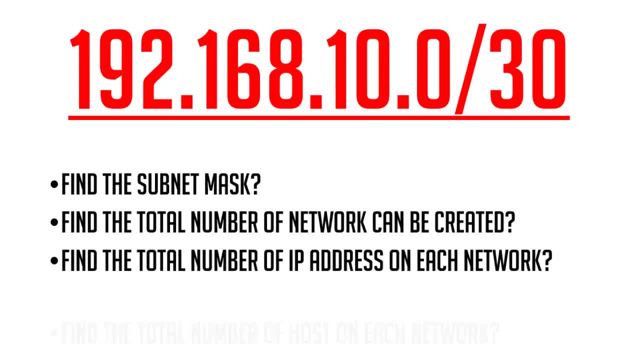 address on each network and, at last, find the total number of hosts on each network? answer this question in the comment section below. I am waiting for you, guys, and let's see whether you are able to pass the test or not. so, guys, this is all about today. if you enjoyed watching this video and please hit the 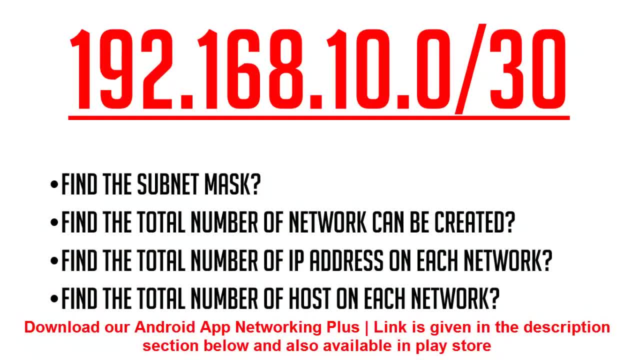 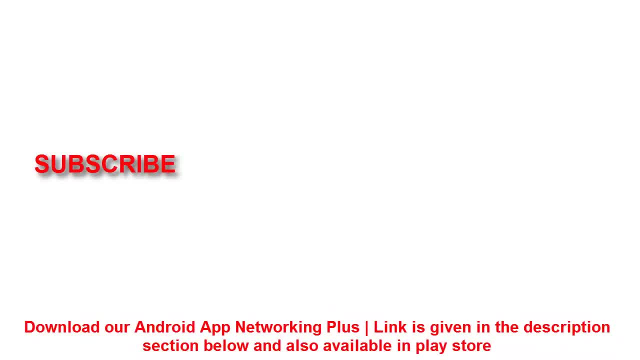 like button and for more interesting tech videos like this, please hit the red subscribe button and also press the bell icon for regular update. thanks for watching you.